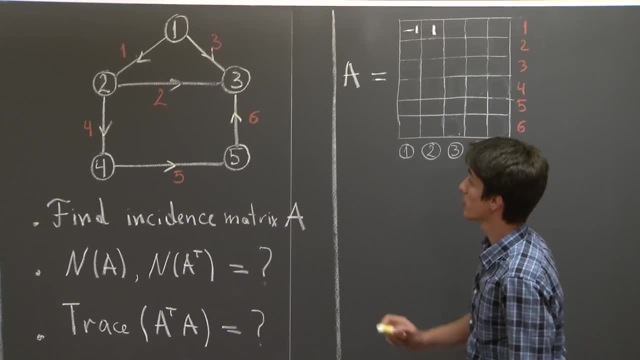 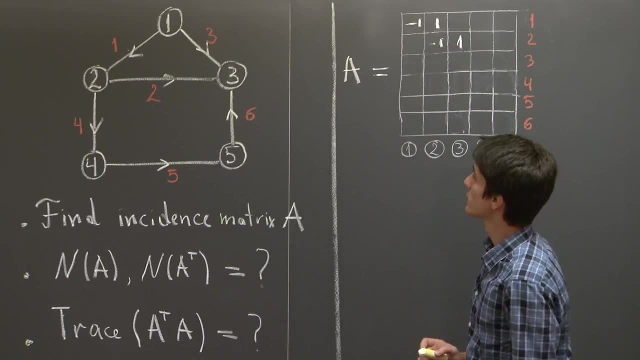 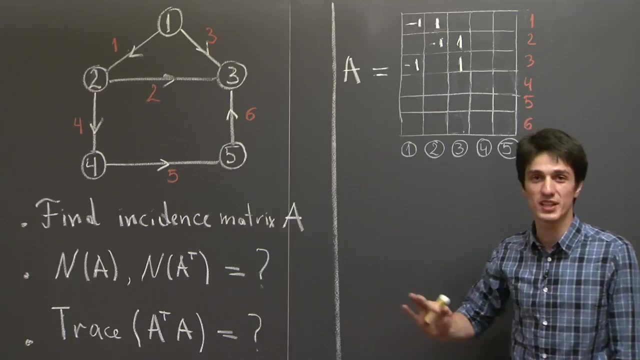 Then edge number two. it connects node two to three, so negative one one. Edge number three connects node one to three, so negative one one, And I believe you get the picture right. So I'm just going to fill out the rest of the entries. 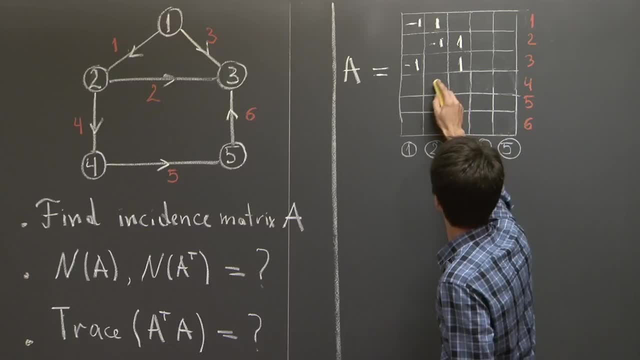 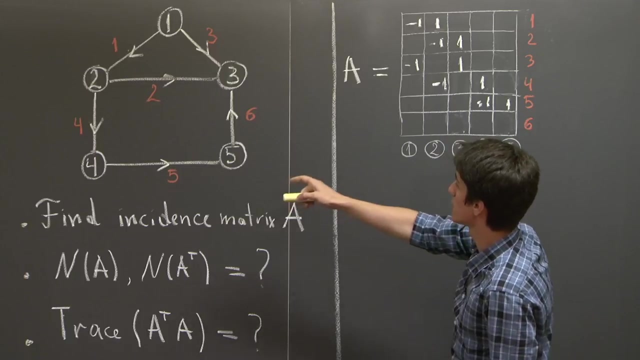 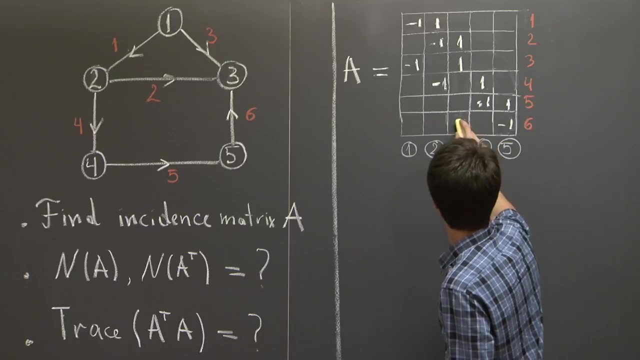 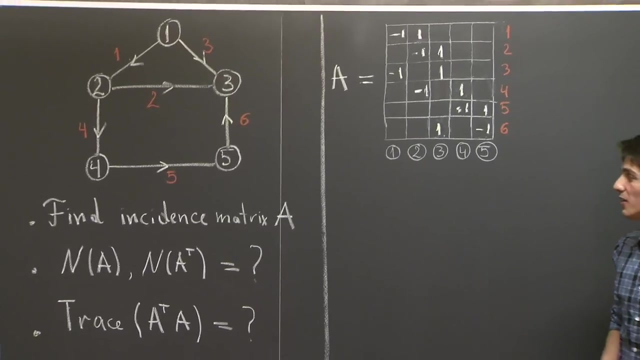 All right, four is negative, two negative, one, Five is negative, two well negative, four well negative, four and one here, And six is one and one. Okay, so we've constructed the matrix A, Now we'll compute its null space. 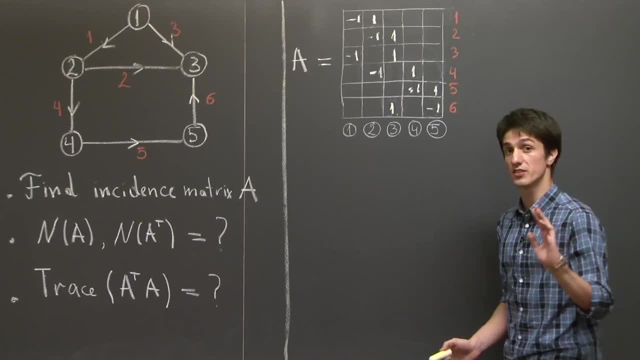 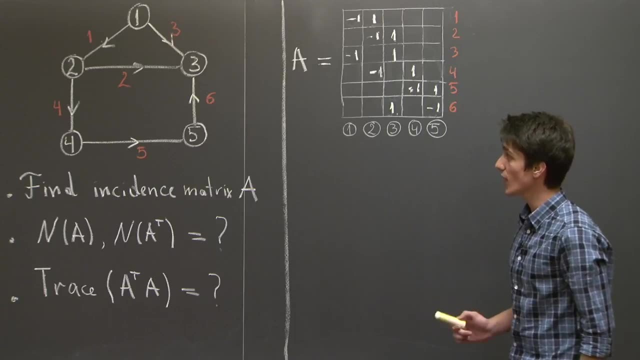 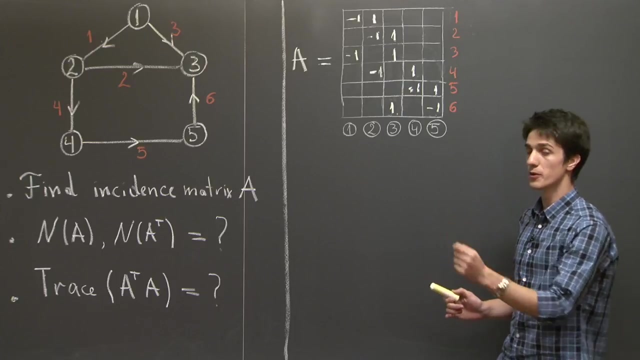 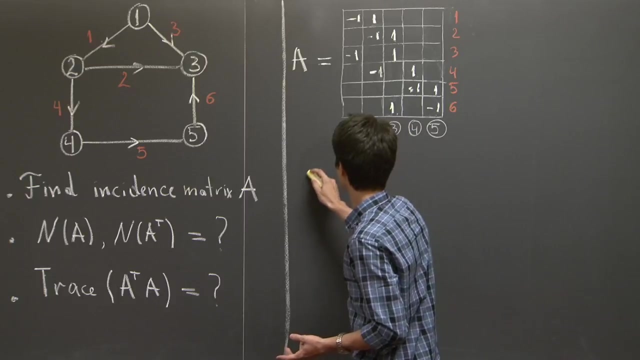 And we're going to do it without performing any row operations whatsoever. So in order to do this, it's helpful to look at the graph as an electric circuit and to assign to each of the nodes an electric potential. If we collect all the electric potentials in a vector x, 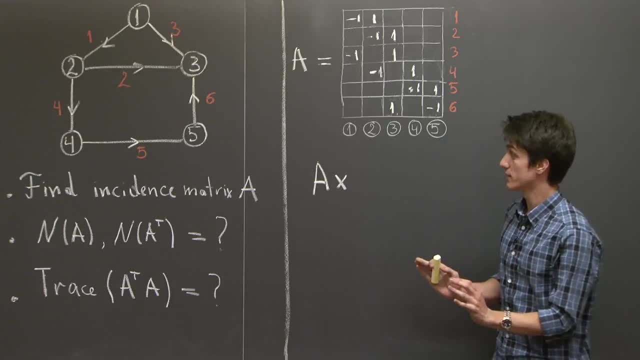 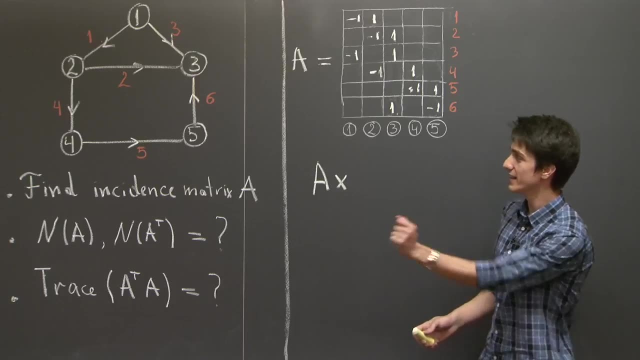 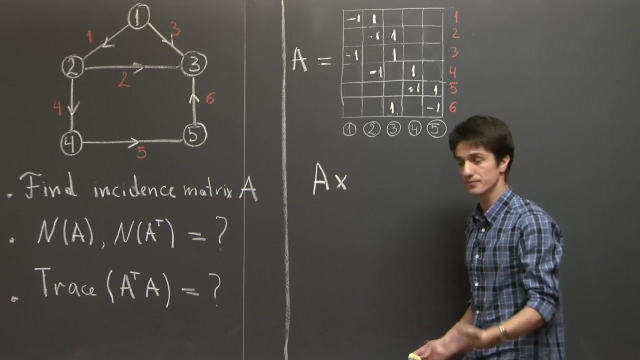 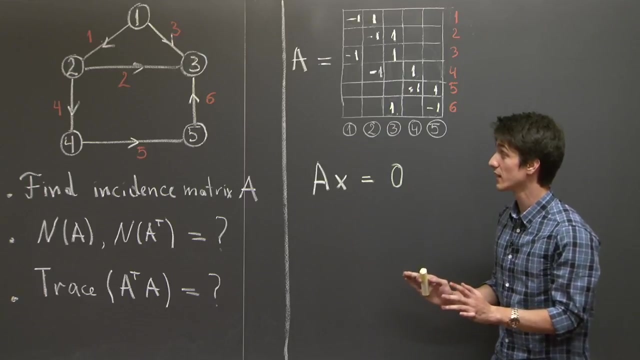 then A times x is a vector with as many entries as there are edges and gives precisely the potential differences across the edges of the graph. Okay, so then, if A x is to be zero, this means that across the graph, like across all the edges of the graph, 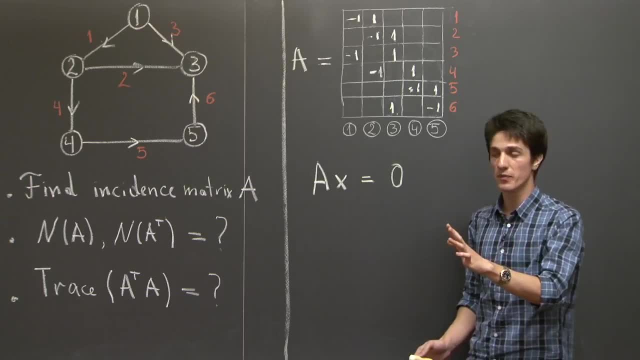 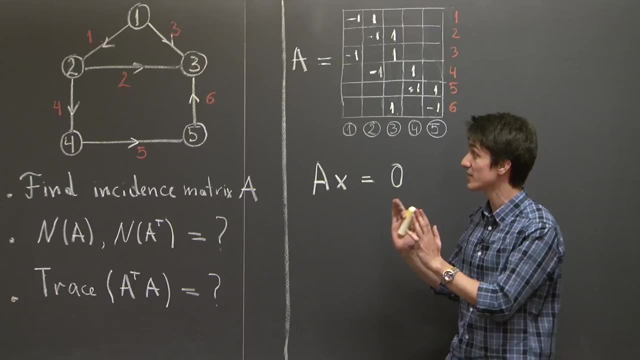 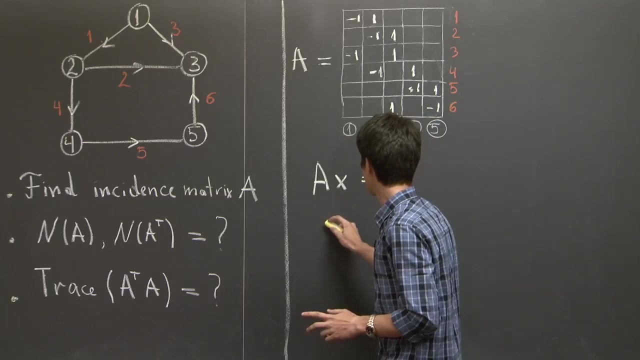 all potential differences are zero. Therefore, all the potentials at all the nodes need to be equal to a constant number. So therefore, we conclude that the null space of A is spanned by constant one. Okay, There are five ones here. 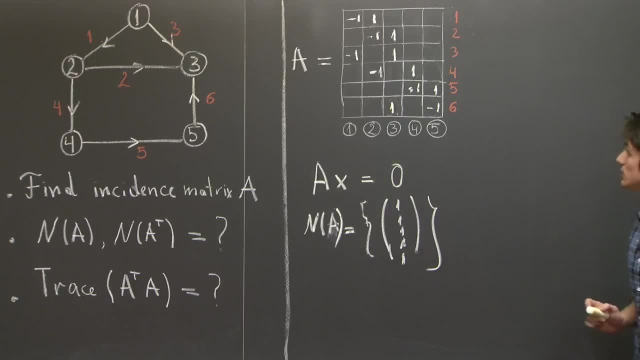 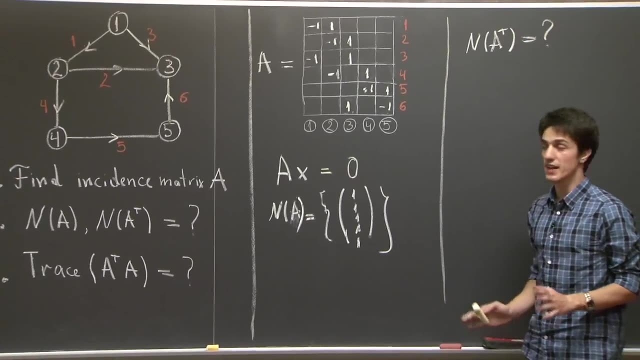 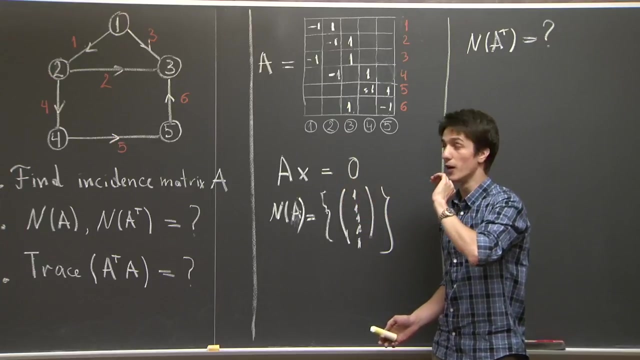 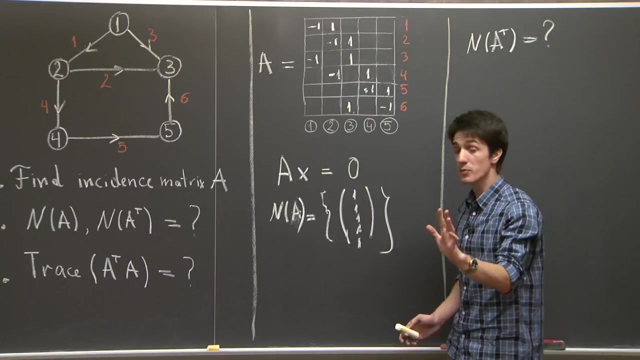 corresponding to the five nodes. Now, what about the null space of A transpose? Adopt this analogy with electric circuits, but this time we're going to look at currents flowing across the edges of the graph. So, Oh, and we're going to adopt the following convention: 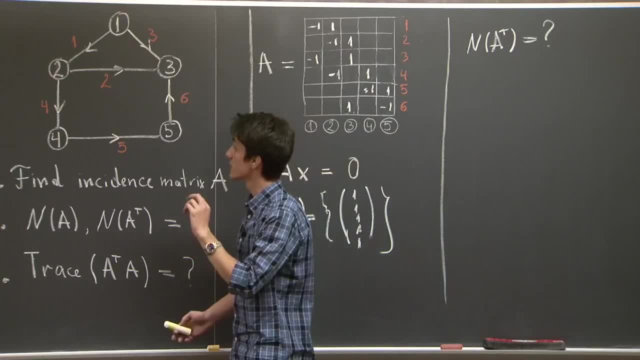 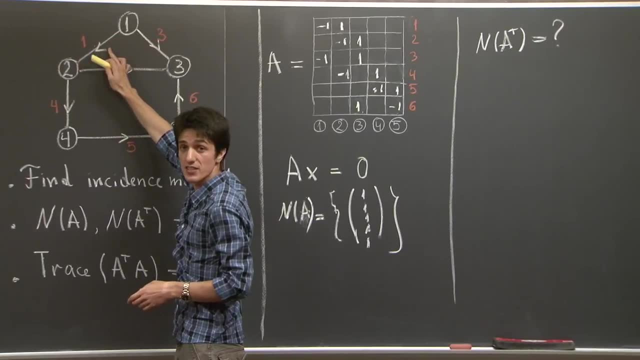 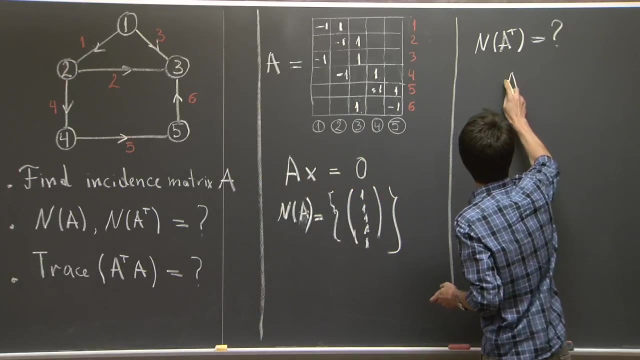 for the currents. So a current is going to be positive if it's if it's if it flows in the direction of the edge, and negative if it flows in the opposite direction. Right, So then, what is A transpose y? 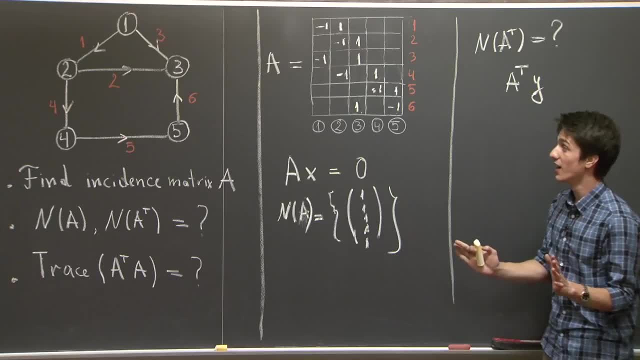 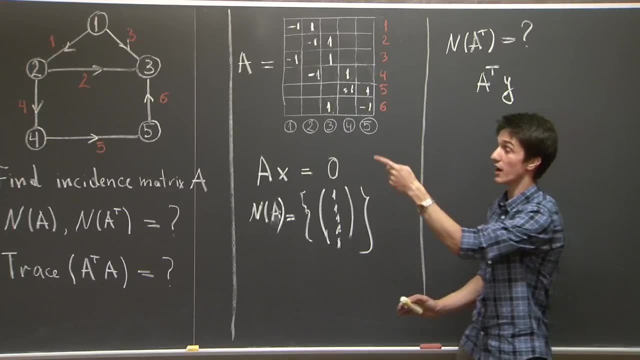 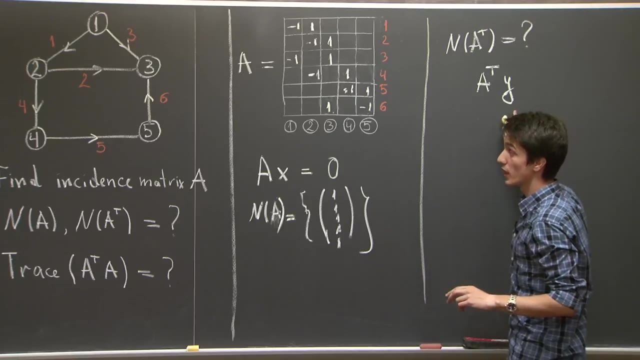 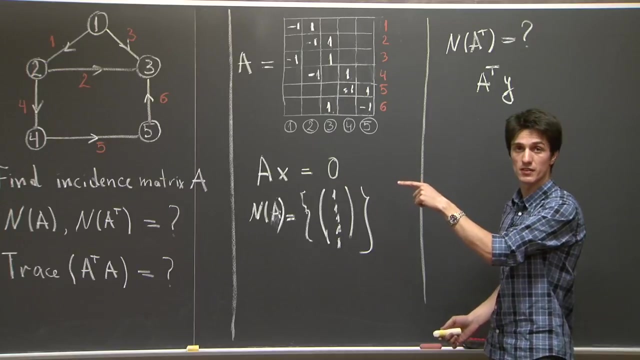 where y is a vector with which which each of whose entry is a current on the edge. Well, it's precisely. the entries of A transpose y are precisely equal to the total current flowing through each of the nodes of the graph. 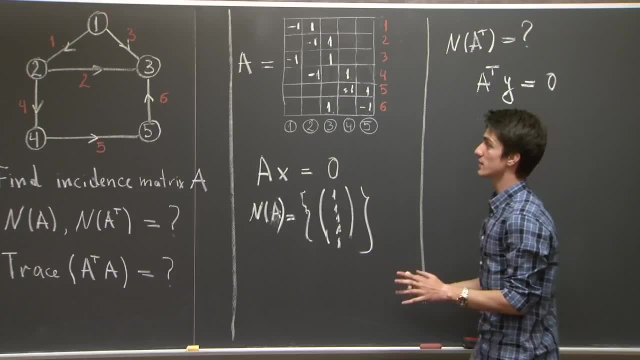 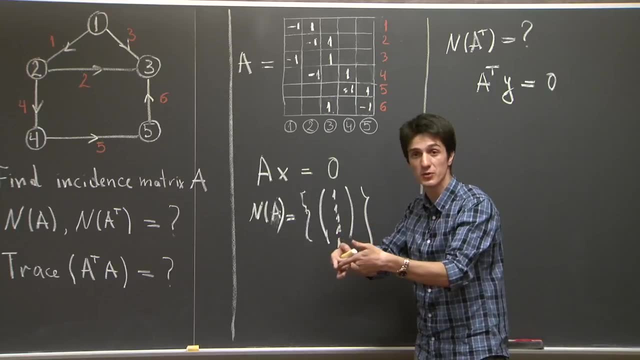 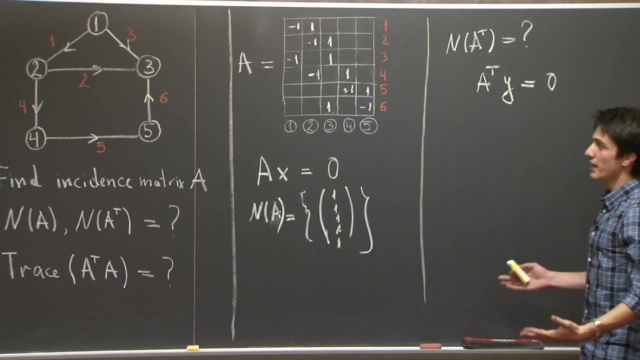 So A transpose y being equal to zero means that there is a balance in the circuit, that the currents that flow through into each node equal the current, the currents that flow out of it. Right, And it's fairly easy to find such configurations. 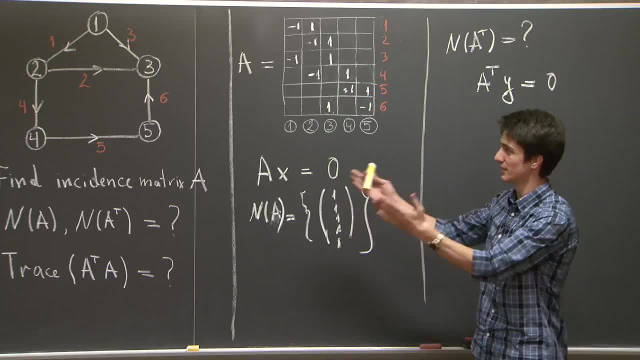 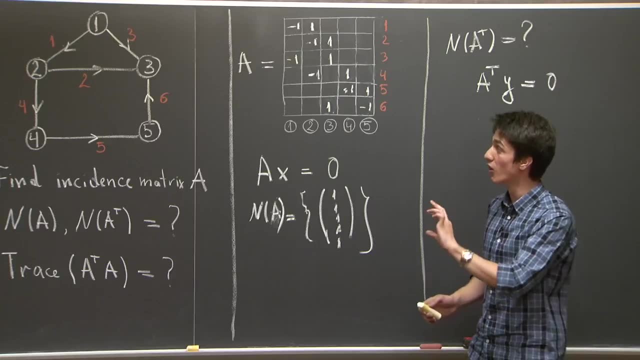 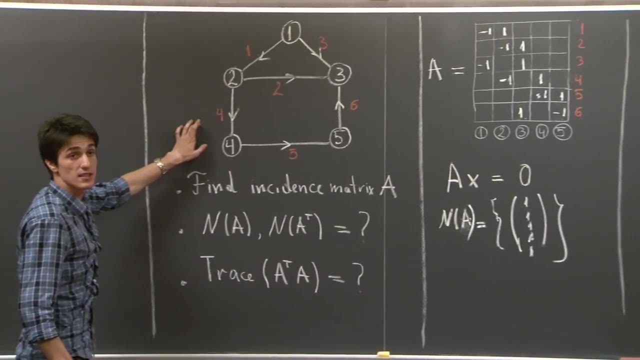 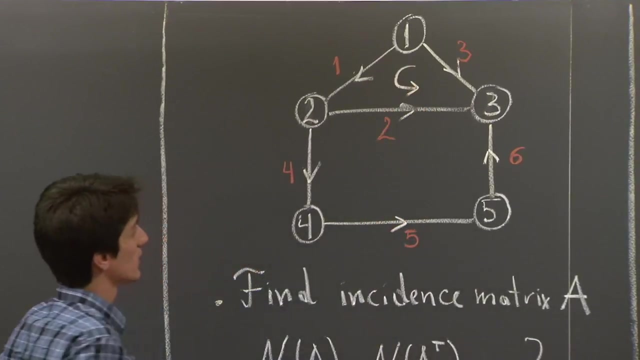 of currents that satisfy this balance equation. We do it by flowing around loops of the graph. So you see, this graph has three loops. The first one is this triangle Up there, The second one is the square, And I'm just 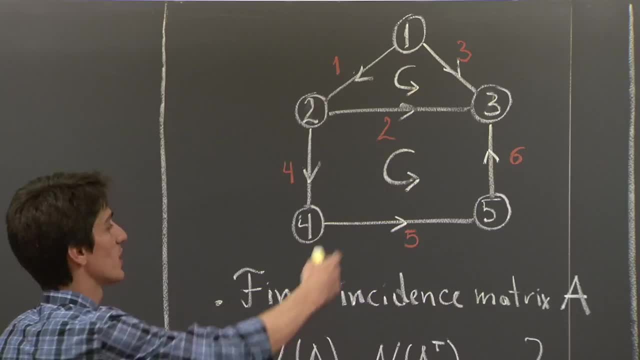 by this, this curled direction, I'm signifying which in which way I'm gonna take. I'm gonna trace the loop And there is a third loop is along the outer contour of the graph, But in fact the third one, 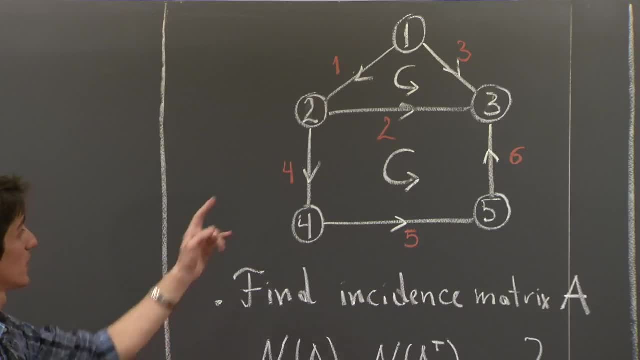 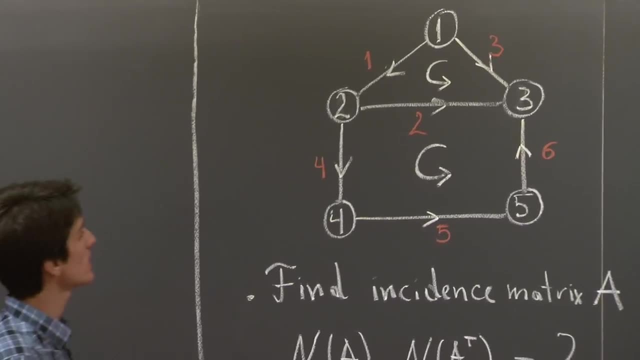 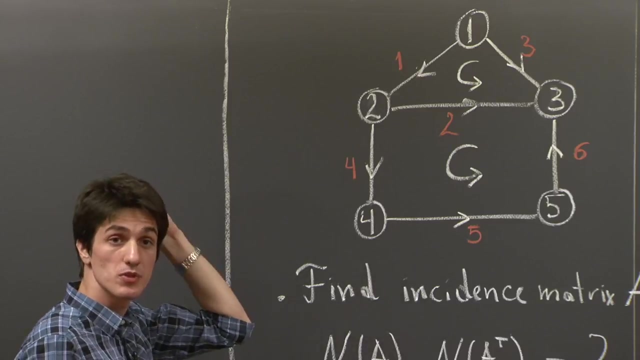 can be thought of as a superposition of these two, And I'll I'll explain why in a second. So let's, let's figure out, yeah, the configuration of, of currents, that that balance these loops. So if we flow a current, 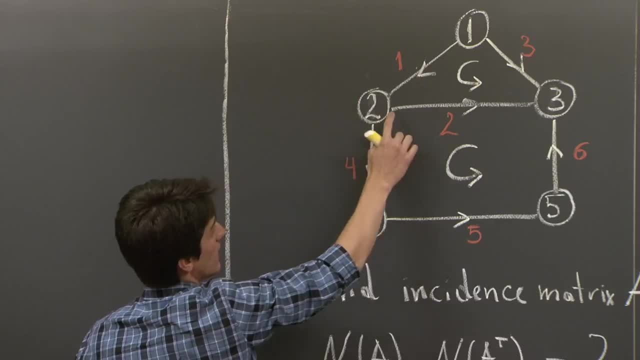 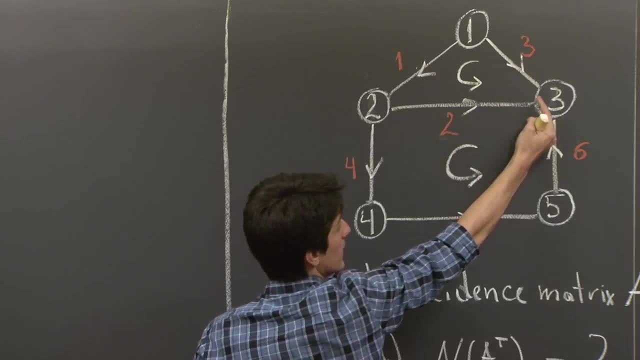 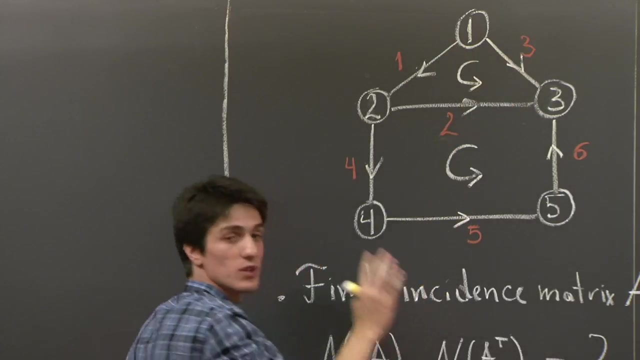 one from one to two, and then flow a current of one along edge two from two to three, and then we flow a current of negative one. mind that the direction is opposite to the direction of the loop. then we're gonna have 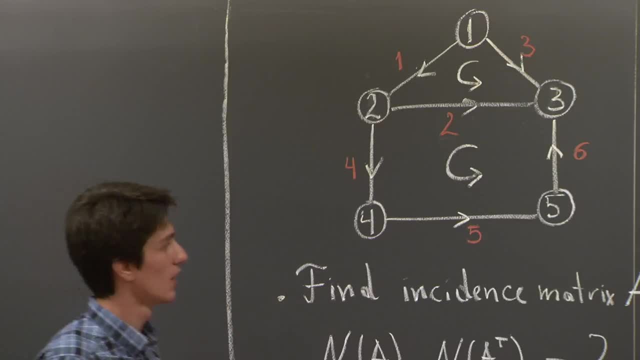 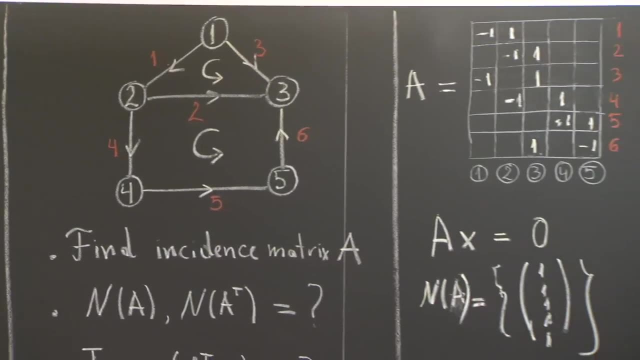 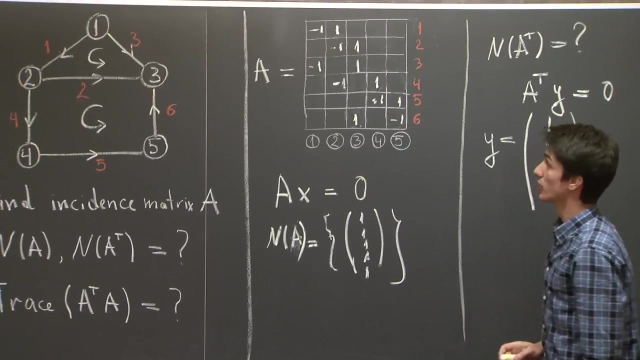 a balanced configuration of currents. So let me write this down, The following configuration: So one along edge one, one along edge two and negative, one along edge three and the rest zero is a solution to A transpose Y. 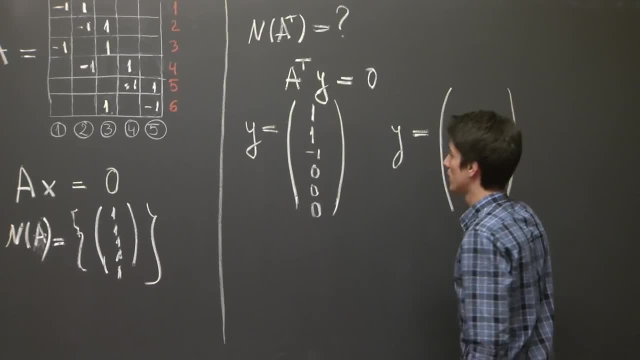 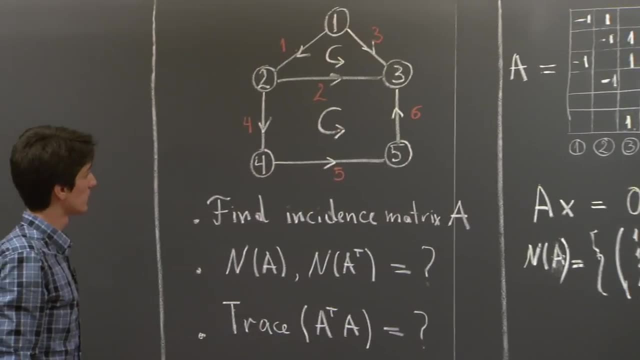 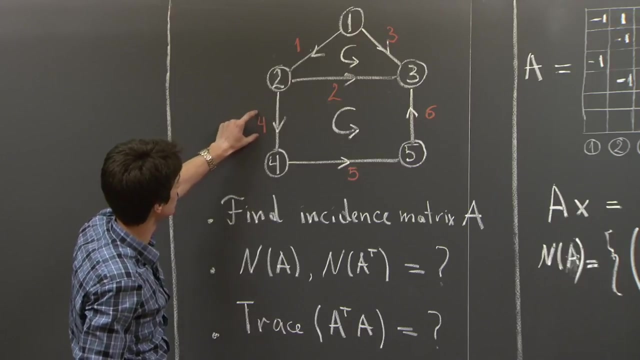 Let's see what solution we get by flowing around the loop in the square. Well, we get a one along. we flow. a. current of one along edge four. current of one along edge five. current of one along edge six. 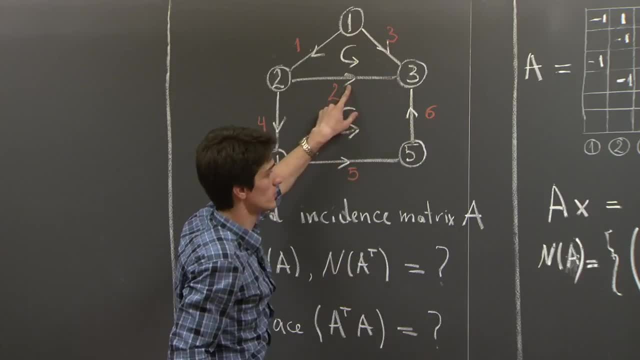 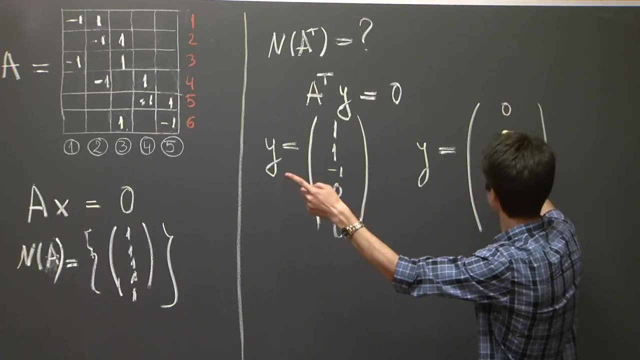 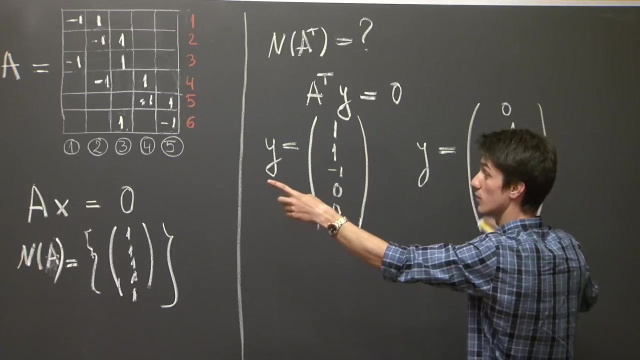 and current of negative one along edge two. So let's be careful. So there was zero then along edge two, was negative one along three, zero along four, one along five, one along six one. 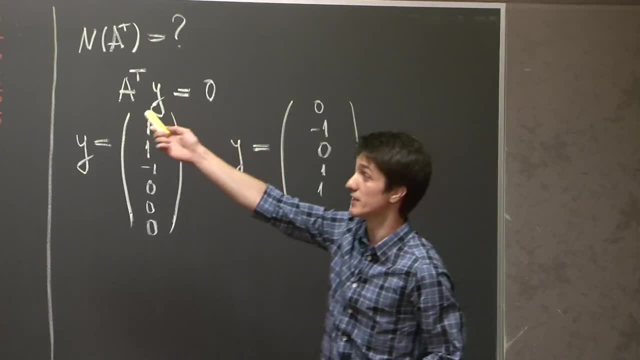 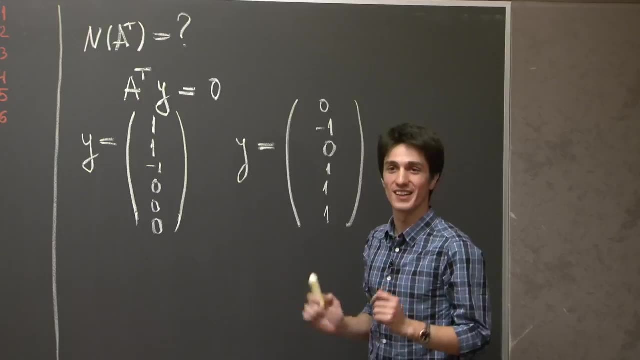 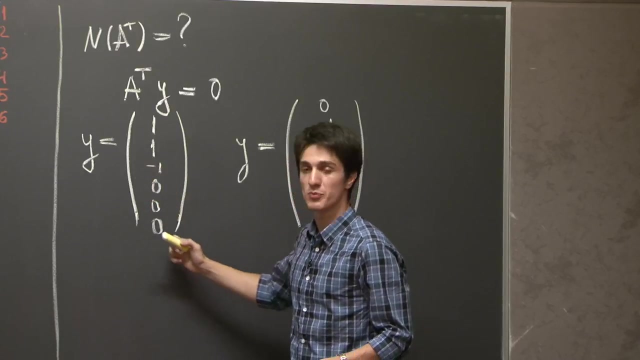 Now we can do the same thing with the, the big loop, and produce a vector corresponding to it, And I I prompt you to do it, But what you'll see is that the vector that you get is precisely a sum of these two vectors. 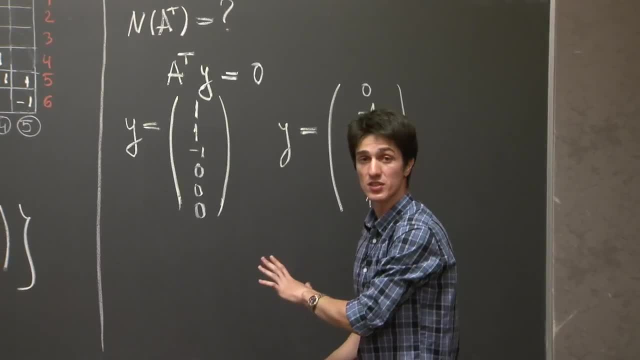 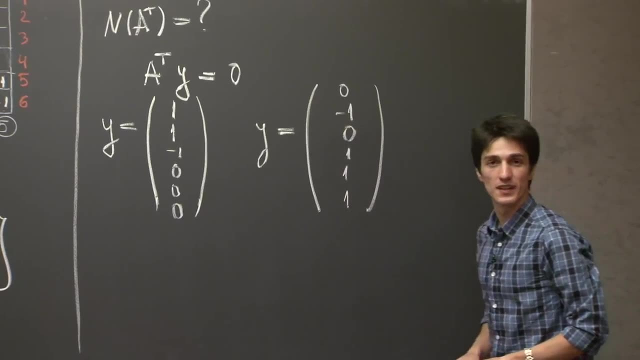 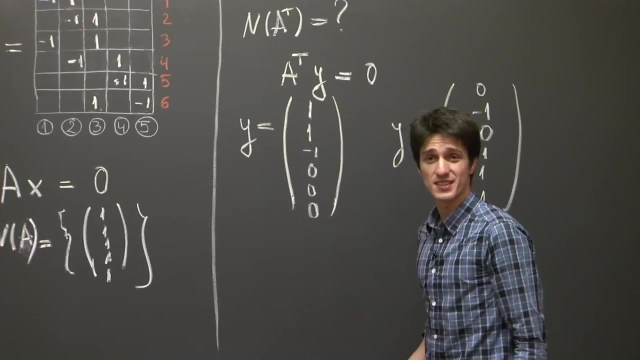 It's a superposition of. in a way, the big loop is a superposition of the small loops. Okay, So we figured out what the null space of A transpose is, And now let's concentrate our attention on finding the trace of A transpose A. 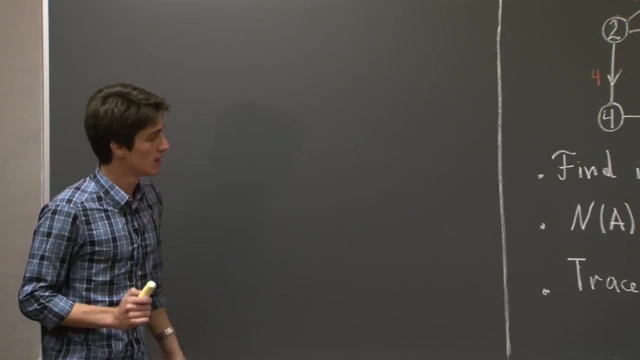 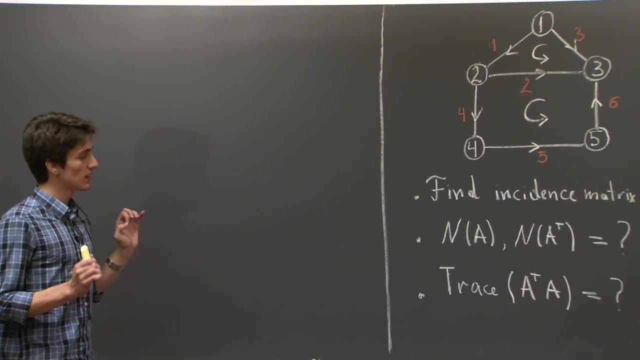 I'm gonna do it right here. So the trace of a matrix is the sum of its diagonal entries, And let's- and we've seen this many times already- that the diagonal entry of the diagonal entries of A transpose A. 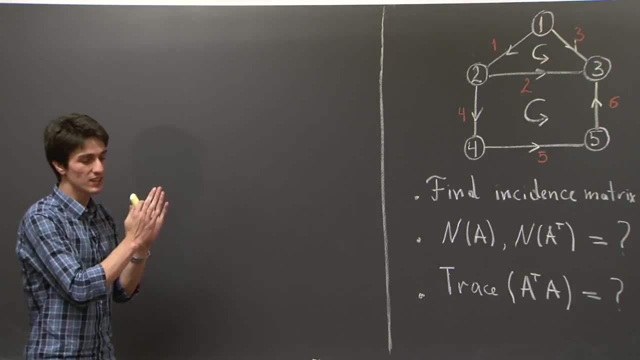 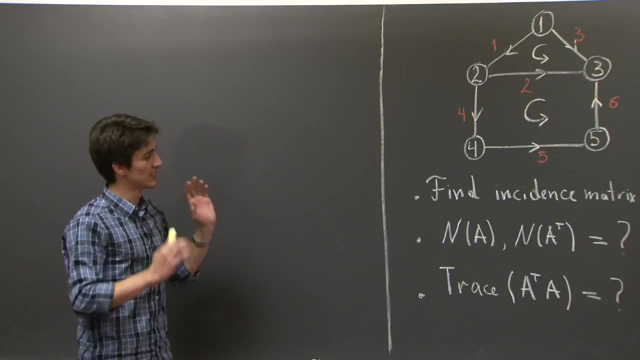 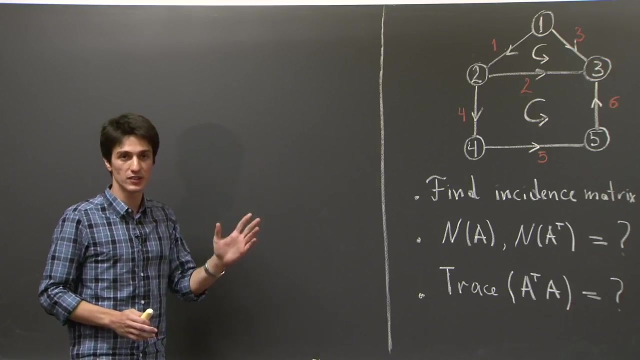 are precisely the magnitude squared of the columns of A. Okay, So the one-one entry is the magnitude squared of the first column, the two-two entry is the magnitude squared of the second column, and so on. Now, what is the magnitude squared? 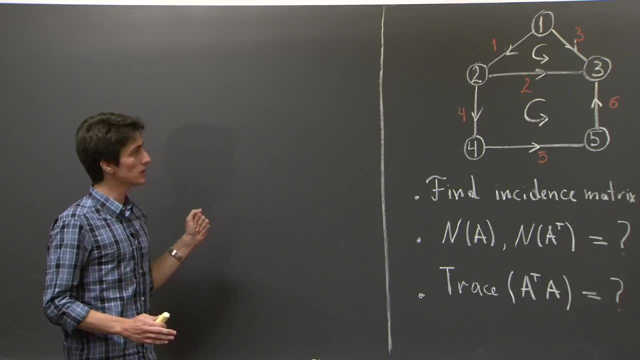 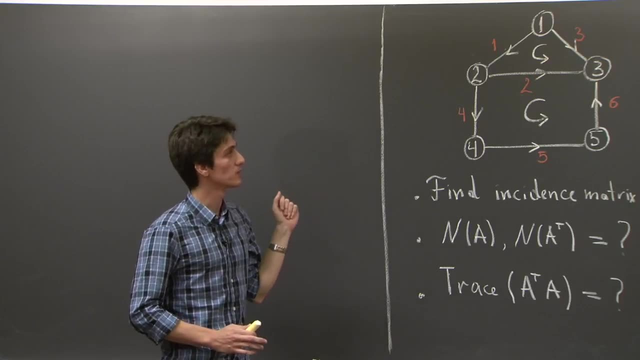 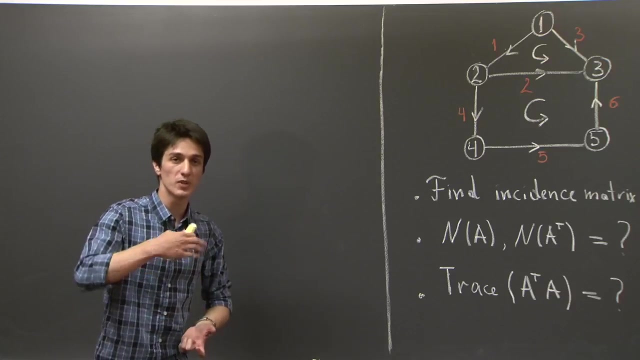 of a column of an incidence matrix. Well, each column of the incidence matrix is either: well, sorry, each entry in a column of an incidence matrix is either one negative one or zero. So when we square these entries, we get ones or zeros. 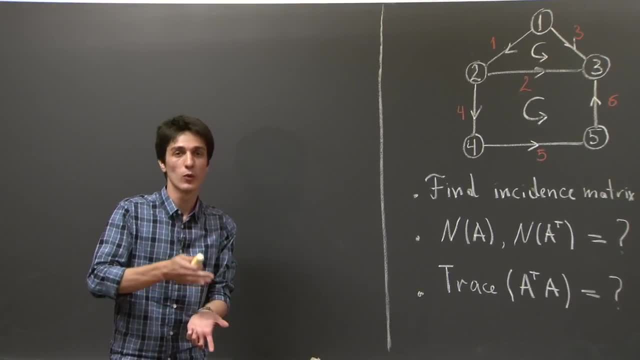 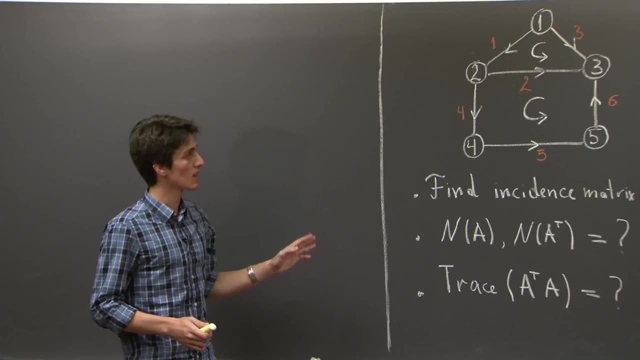 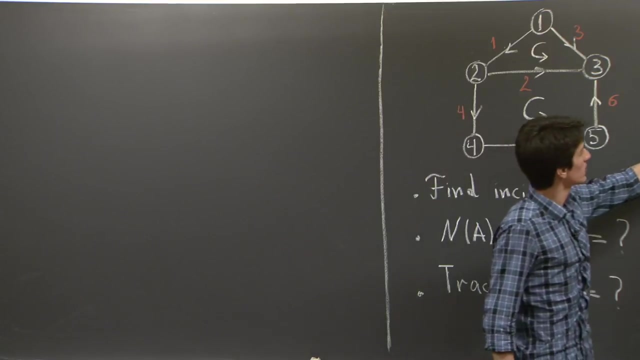 And we add them. when we add them up, we get precisely a number, which is the non-trivial entries in the column. Okay, So the magnitude squared of the column is the number of non-trivial entries in it. But if we go back to the matrix A, 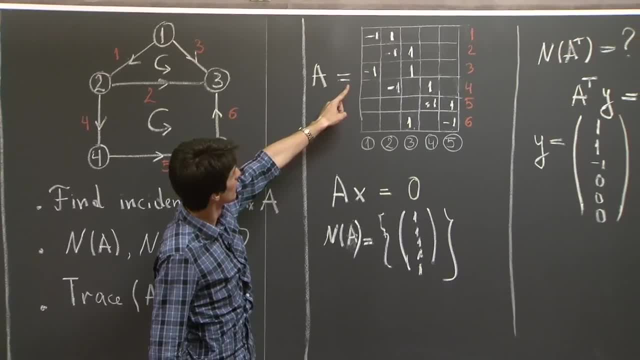 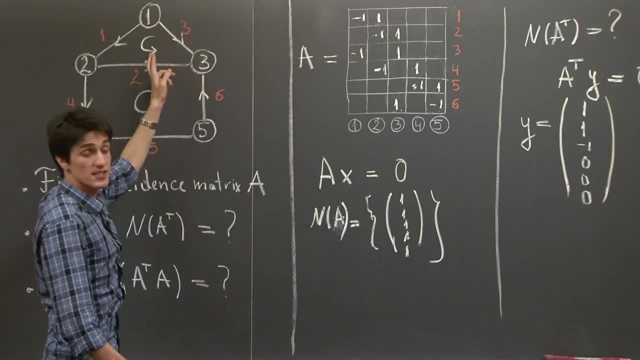 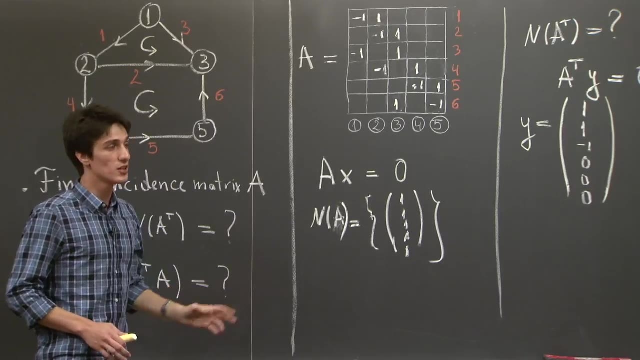 and we count the number of non-zero entries. these are precise. this is precisely the number of edges that connect with the node. Okay, So the number of edges that connects with each node is called the degree of the node In this way. 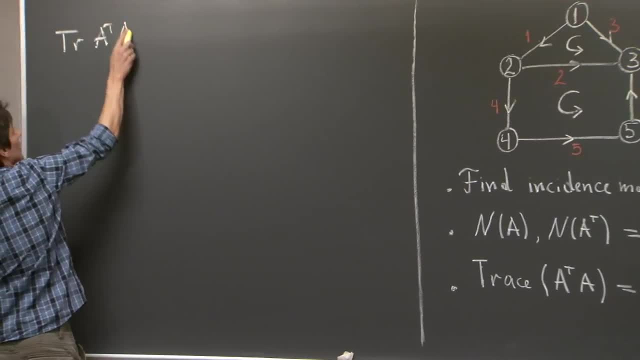 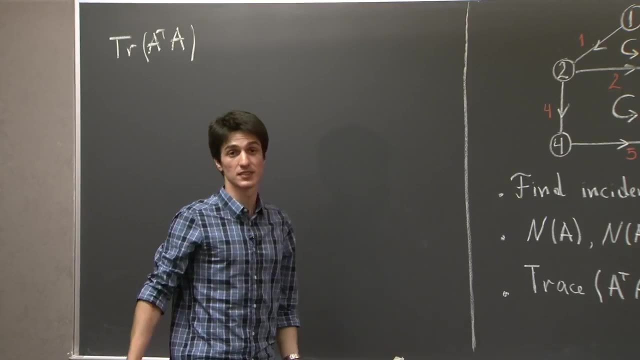 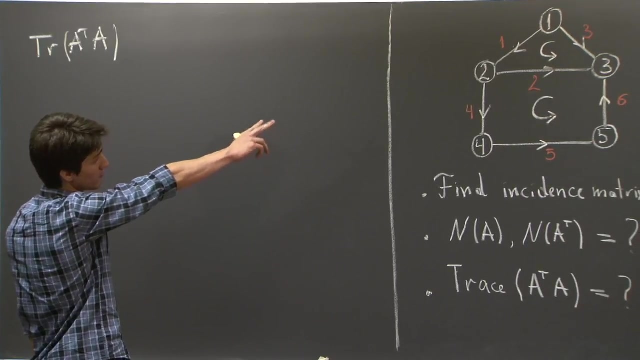 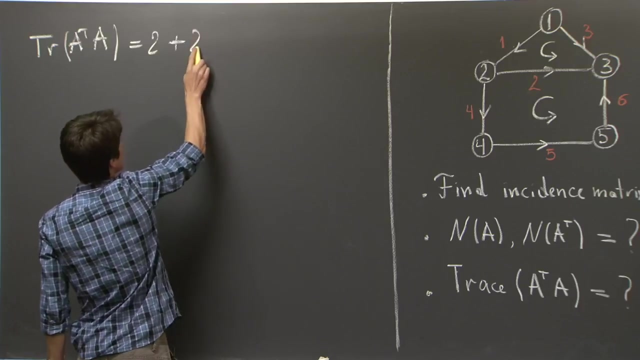 trace of A. transpose A will be just the sum of the degrees of the graph in the picture. So we have one connects one. there are two edges connecting to one, So two plus two edges connecting to two plus- sorry- three edges connecting to two.